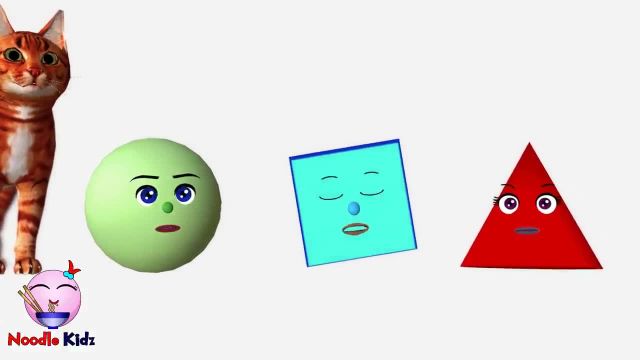 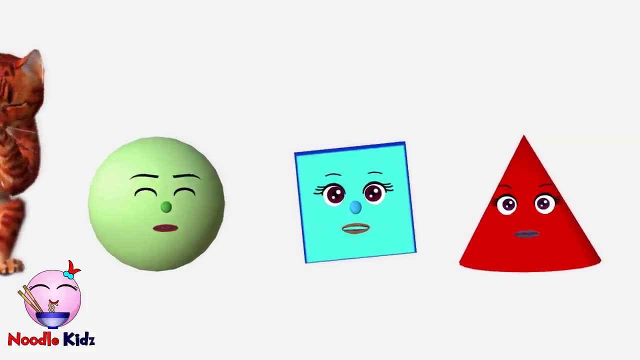 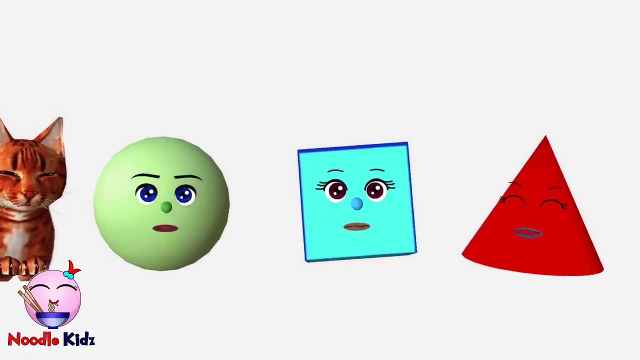 That is correct. Sphere here does not have a flat surface. It has only one curved face. Every 3D shape has one or more flat surfaces, with the exception of sphere here, Just like me, Even though I look like I have only one curved face. 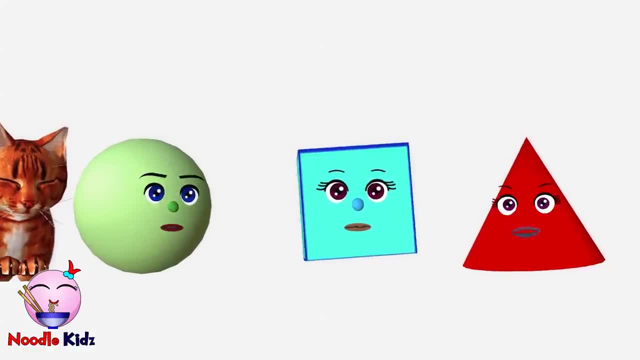 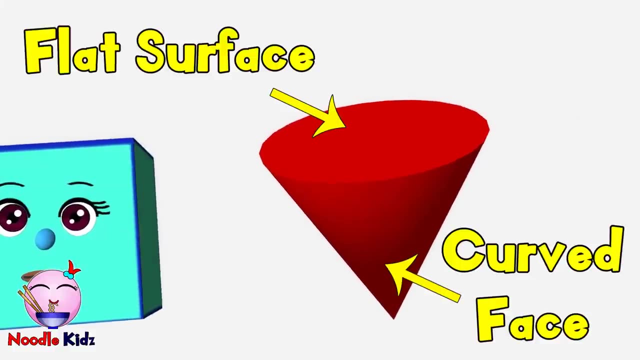 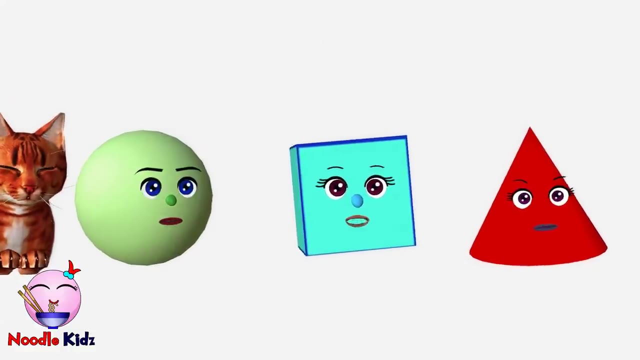 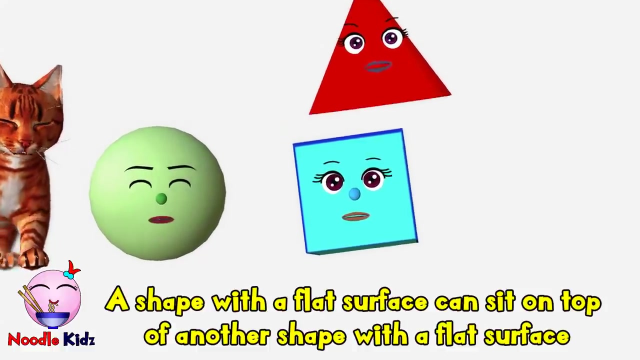 I do have one flat surface. Hold on, let me do a flip There. This is my flat surface. Interesting, right? Do you know what's the difference between a flat surface and a curved face? A shape with a flat surface can stay still on top of other flat surfaces. 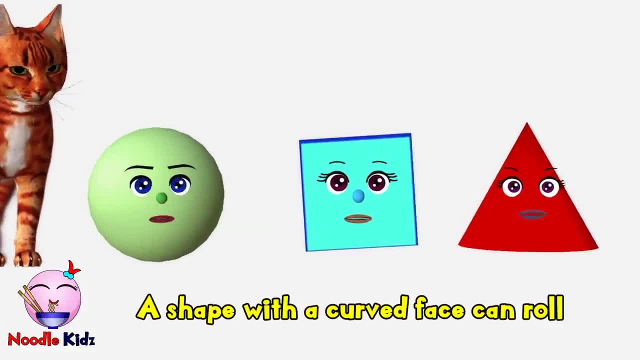 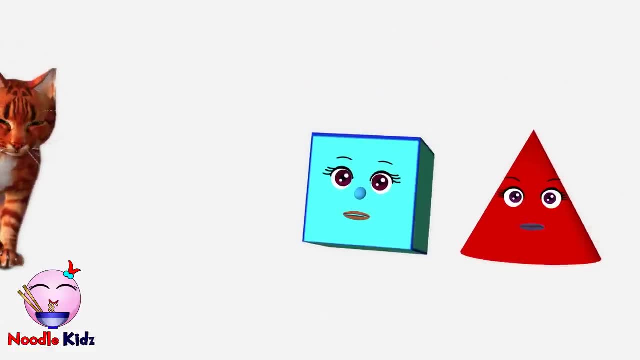 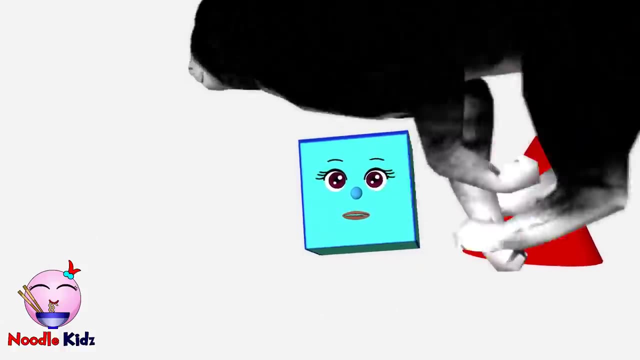 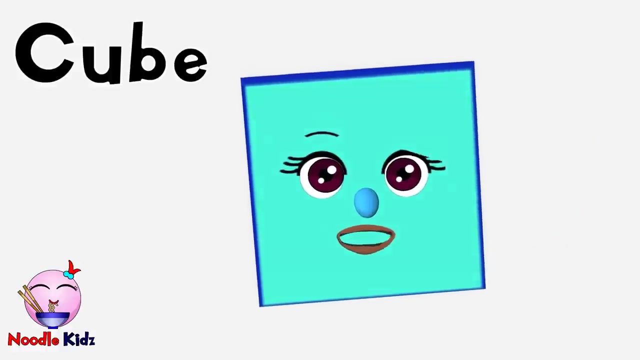 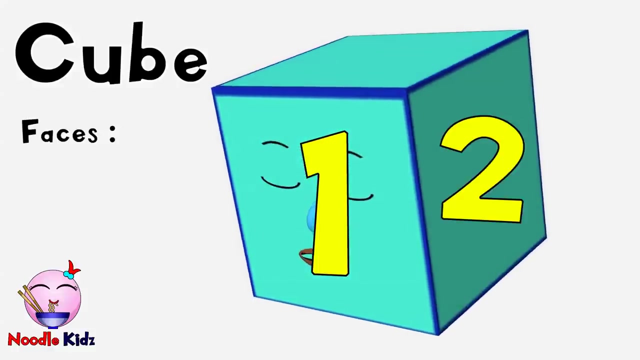 While a curved face could roll away. That is correct. like This, Meow, I don't have a curved face, therefore I cannot roll, But I have many flat faces. Let's count them: 1, 2, 3, 5. 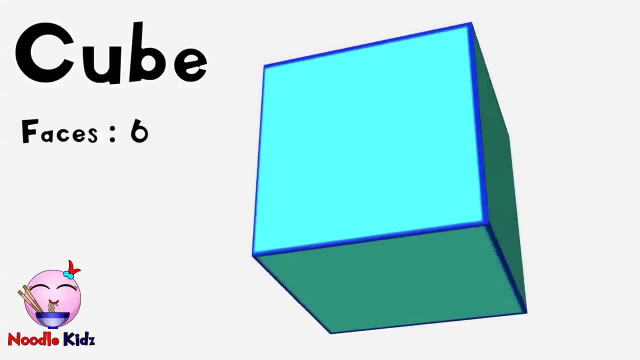 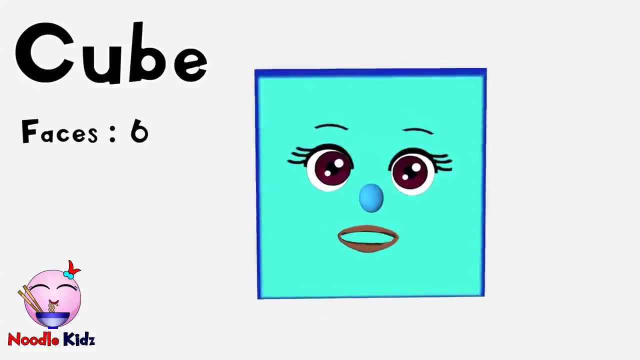 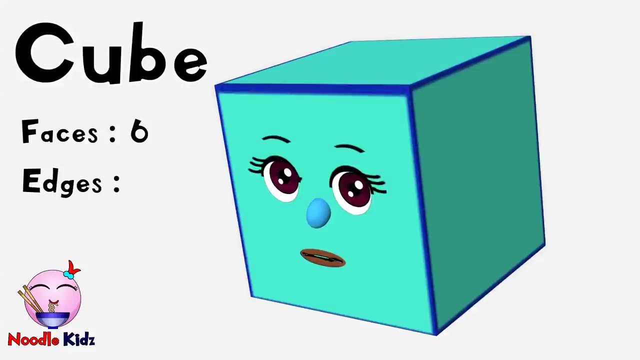 Four, five, six. That's right, A cube has six flat faces. Some 3D shapes also have edges. Do you know what an edge is? An edge is the place where two flat faces meet. Edges are straight. They cannot be curved. Look at this, This is one of my edges. 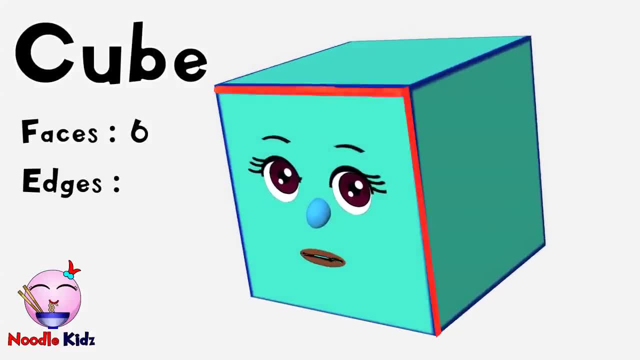 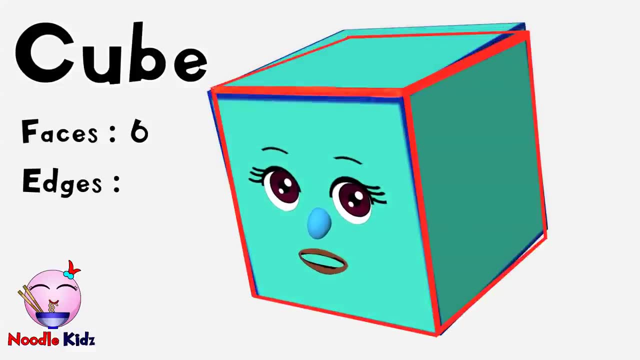 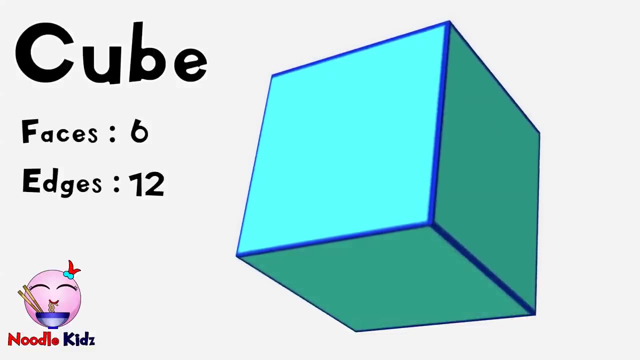 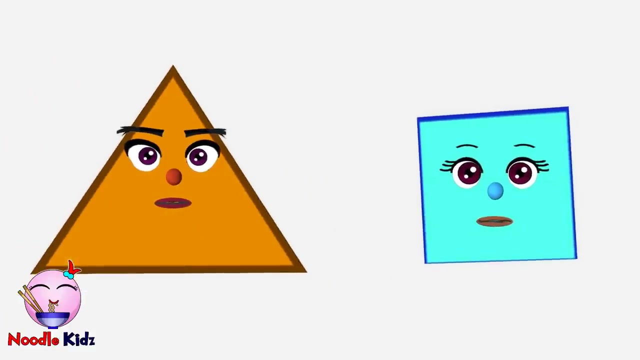 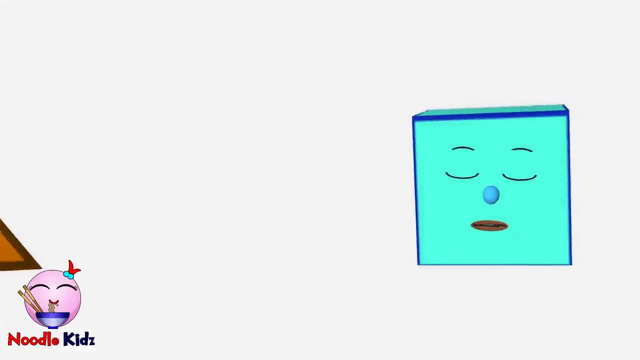 Let's count my edges: One, two, three, four, five, six, seven, eight, nine, ten, eleven, twelve. Yes, A cube has twelve edges. Hey, Don't forget about vertices, Right? A vertex is the place where there are two or more edges meet. 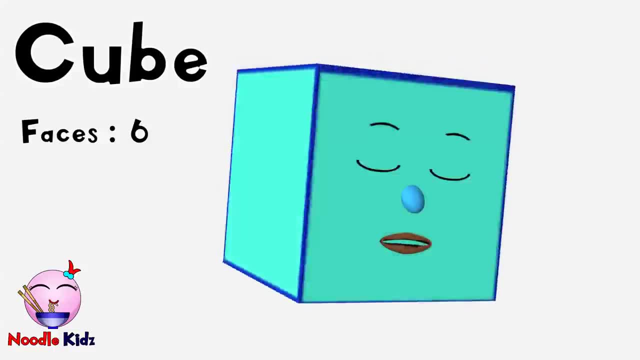 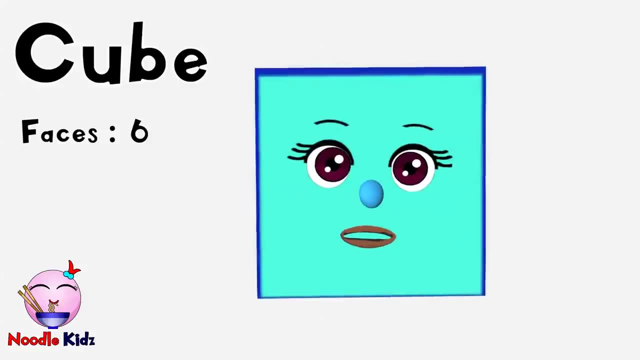 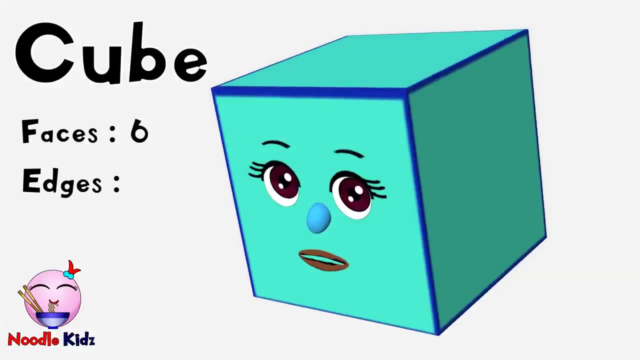 Six, That's right. A cube has six flat faces. Some 3D shapes also have edges. Do you know what an edge is? An edge is the place where two flat faces meet. Edges are straight. They cannot be curved. 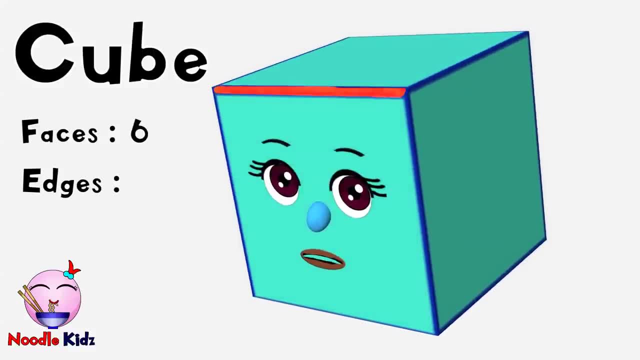 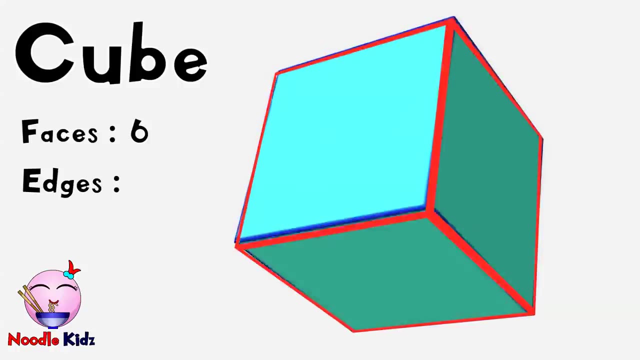 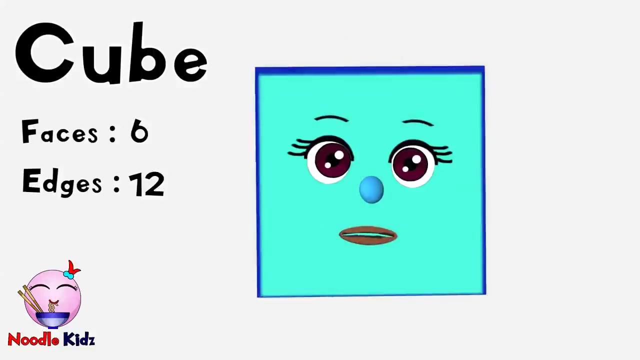 Look at this. This is one of my edges. Let's count my edges: One, Two, Three, Four, Five, Six, Seven, Eight, Nine, Ten, Eleven, Twelve. Yes, A cube has twelve edges. Hey, Don't forget about vertices. 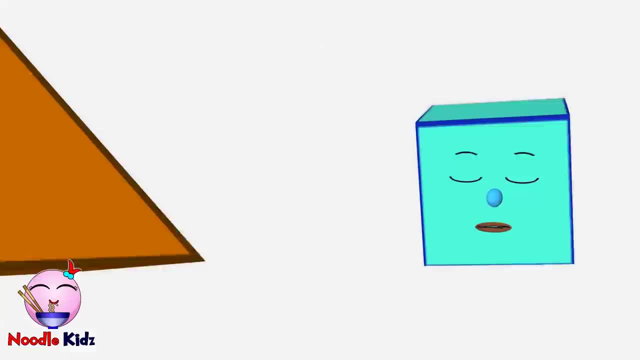 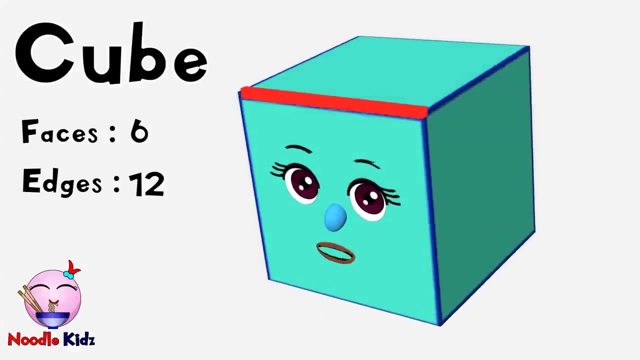 Right. A vertex is the place where there are two or more edges meet. Look at this. This is where my edge one, edge two and edge three meet. This point is called a vertex. I have more than one vertex. They are called vertices. 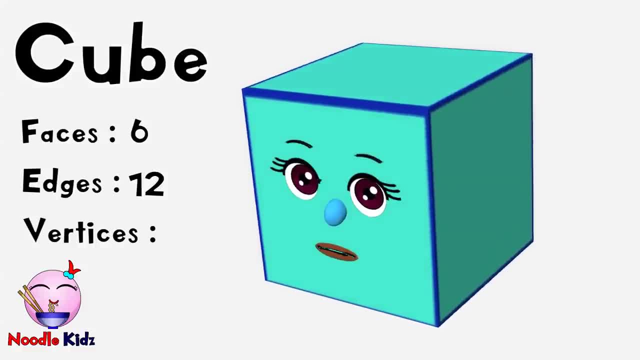 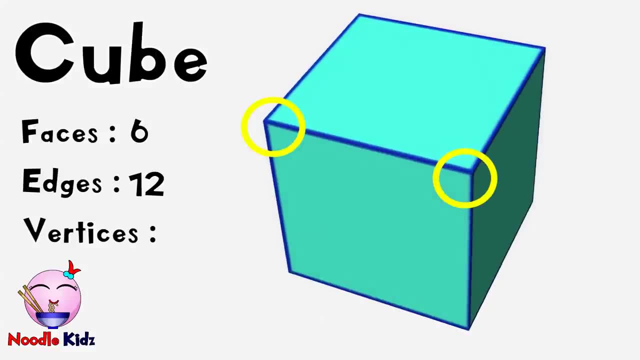 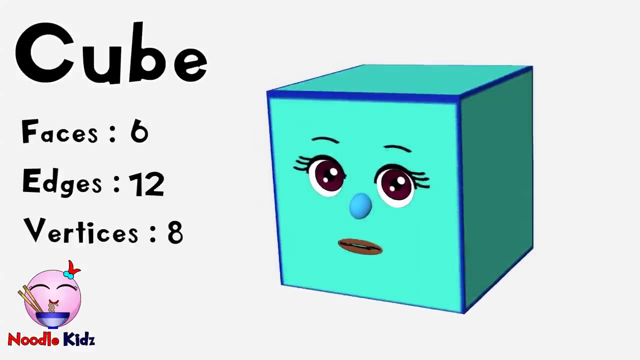 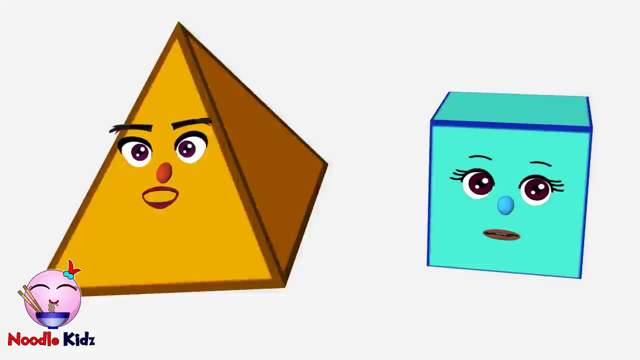 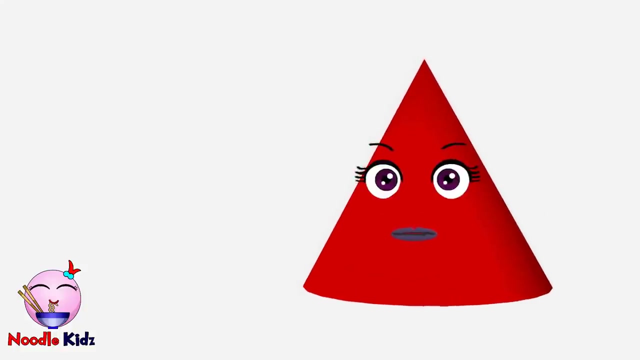 Let's count how many vertices I have. One, Two, Three, Four, Five, Six, Seven, Eight, Yep. A cube has eight vertices. Can you help us identify how many faces, edges and vertices we have? Great, Let's start with me. 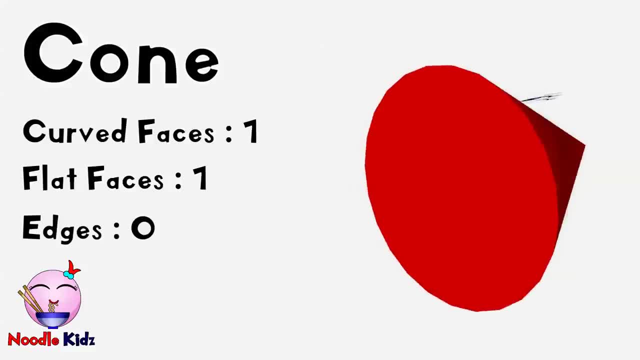 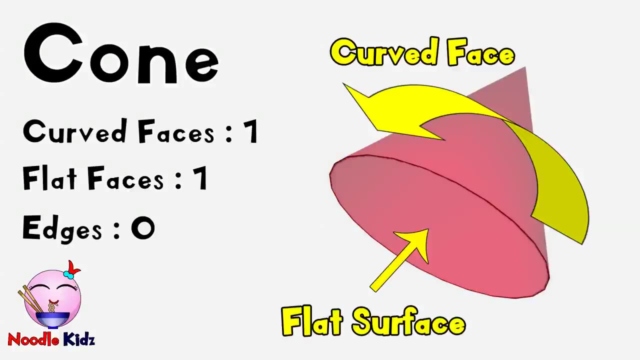 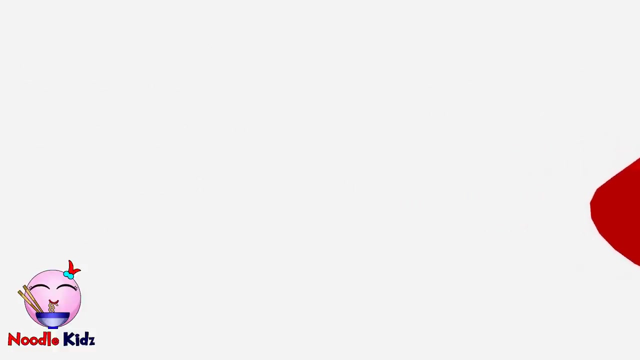 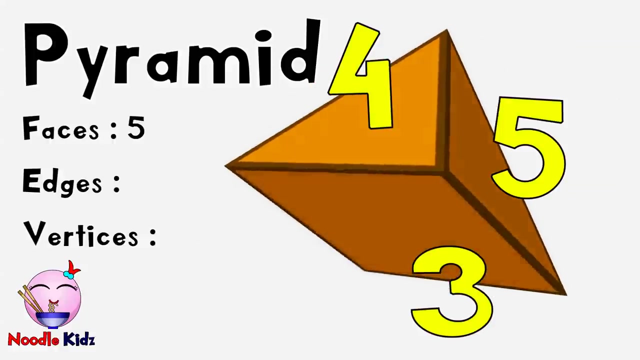 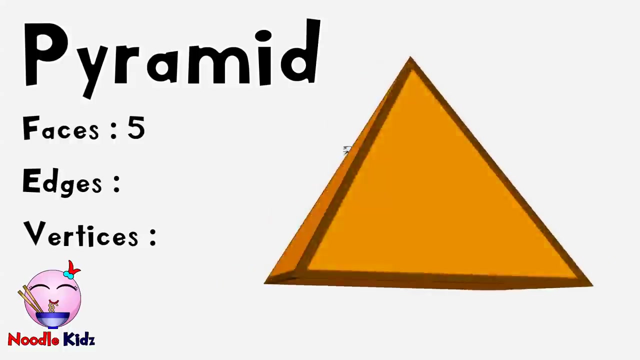 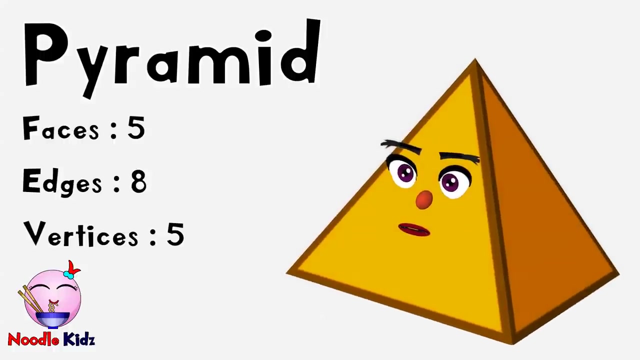 I have one curved face and a flat surface, but I don't have any edges, which means a cone has one curved face, one flat face and zero edges and vertices. Next is me. I am a pyramid. I have one, two, three, four, five faces. I also have one, two, three, four, five vertices, So a pyramid has five faces. 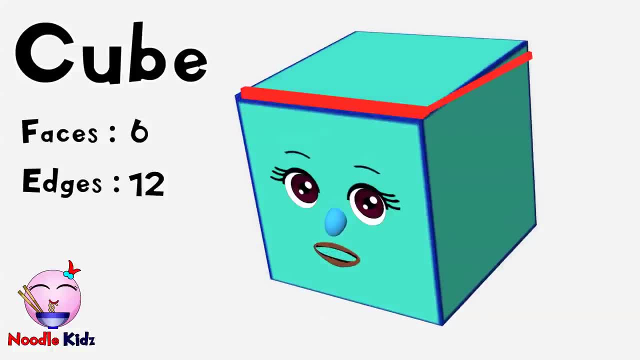 Look at this. This is where my edge one, edge two and edge three meet. This point is called a vertex. I have more than one vertex. They are called vertices. Let's count how many vertices I have: One, two, three, four. 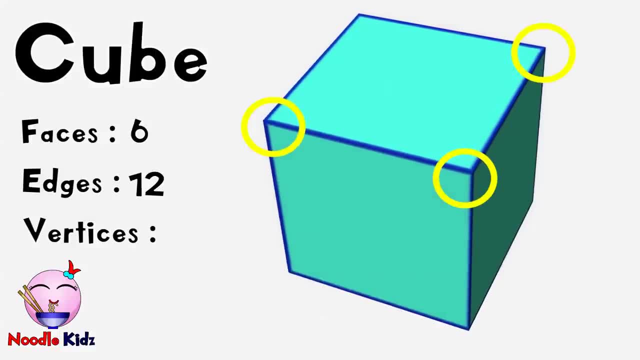 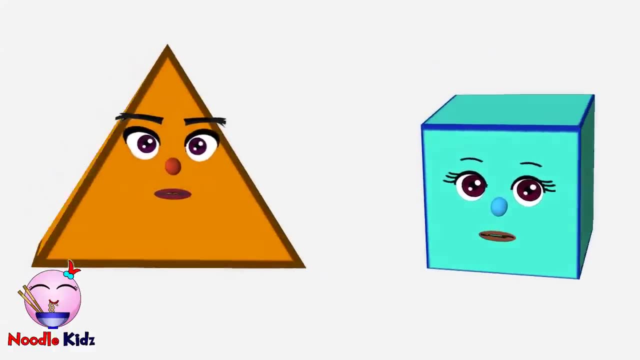 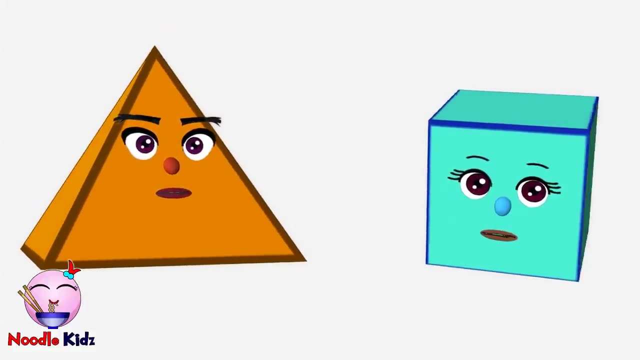 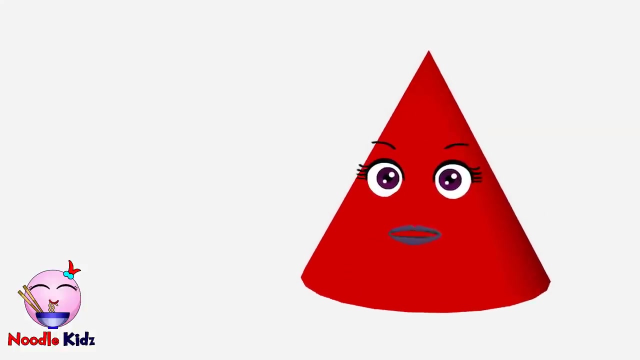 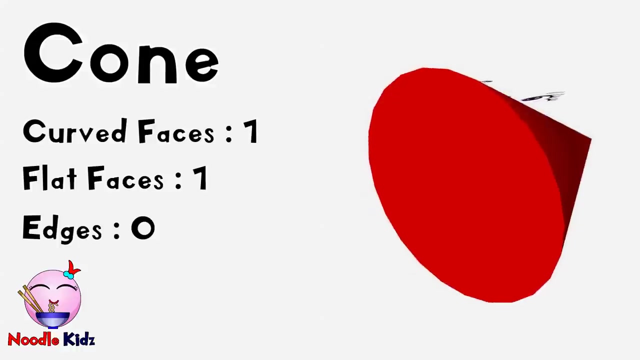 Five, six, seven, eight Yep. A cube has eight vertices. Can you help us identify how many faces, edges and vertices we have? Great? Let's start with me. I have one curved face and a flat surface. 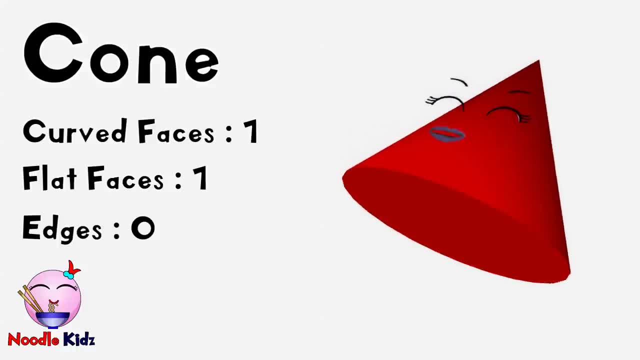 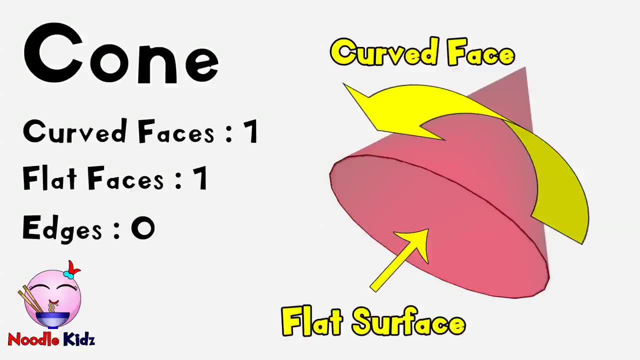 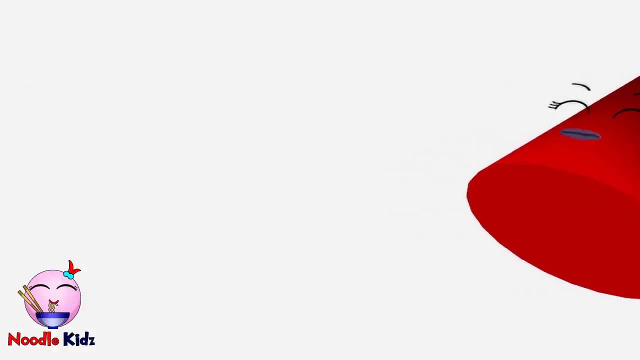 But I don't have any edges, Which means a cone has one curved face, one flat face and zero edges and vertices. One curved face, One flat face, One curved face, One flat face, One curved face, One curved face. 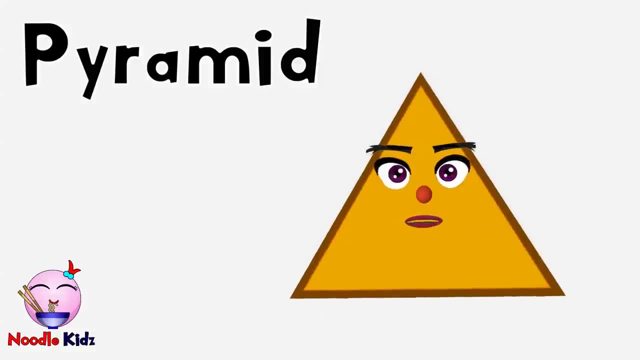 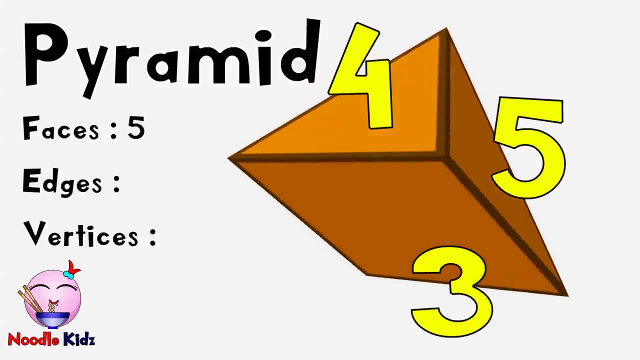 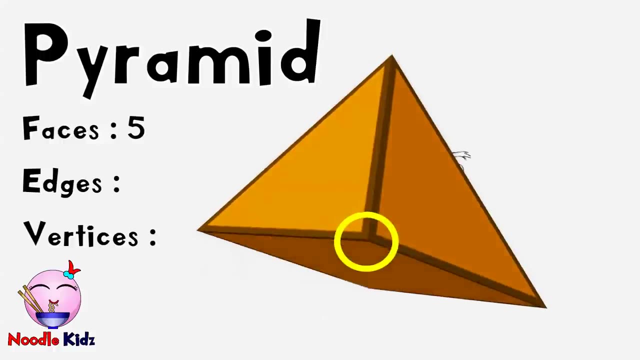 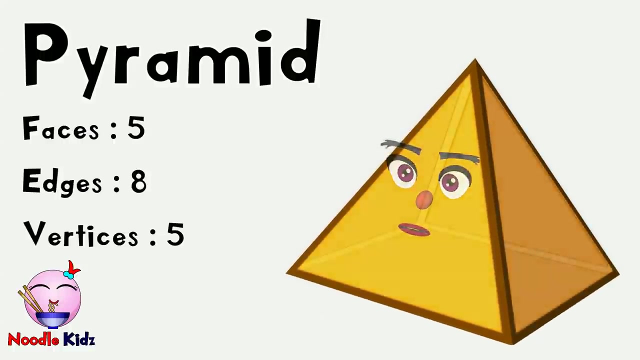 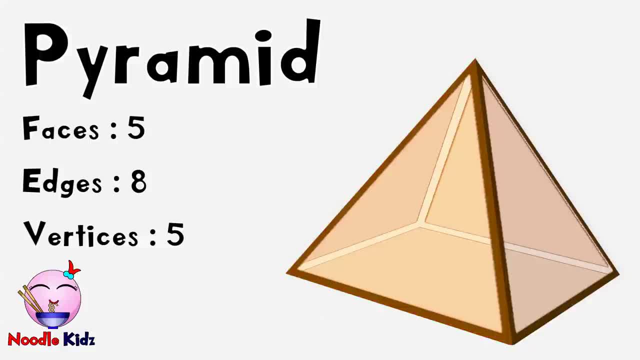 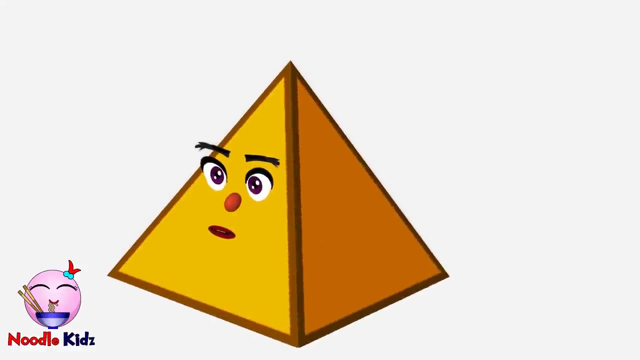 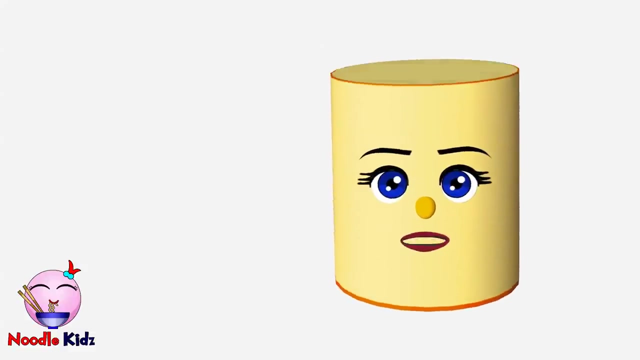 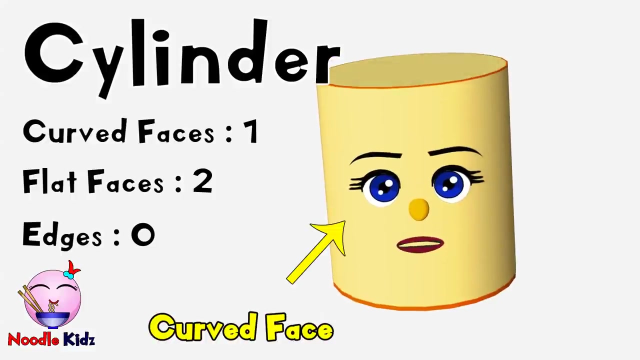 Hủ and I. classics, Eight edges, Five vertices. I'm next. Do you remember my name? Yes, I am a cylinder. Good job, I have one curved face and I have one. two flat surfaces. I don't have any edges, though. 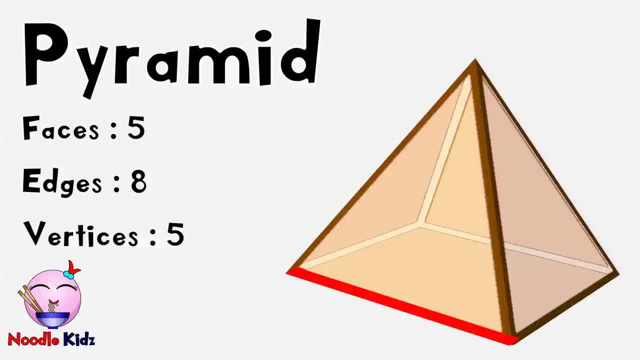 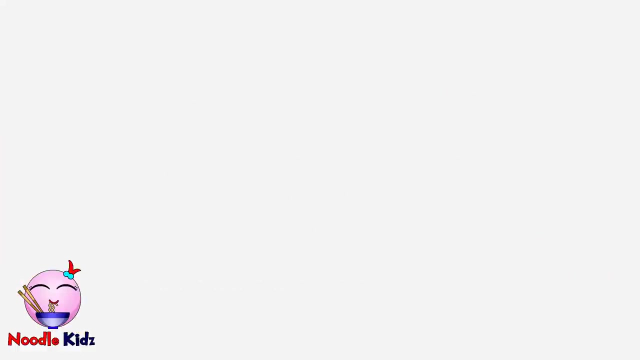 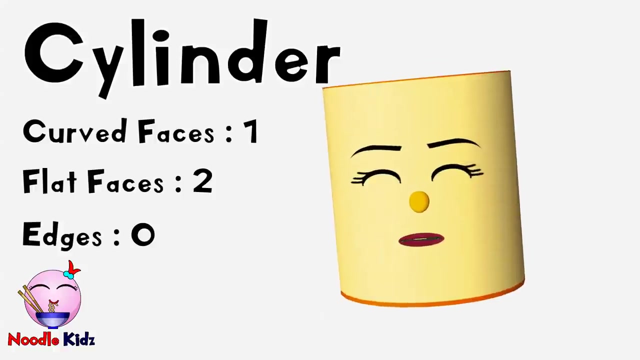 eight edges, five vertices. I'm next. Do you remember mining? Yes, I am a cylinder. Good job. I have one curved face and I have one two flat surfaces. I don't have any edges, though, which means I also don't have any vertices. 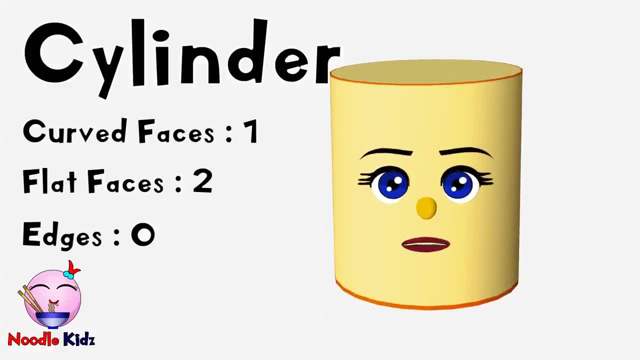 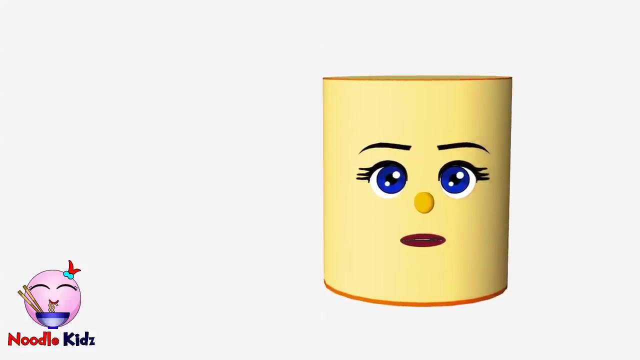 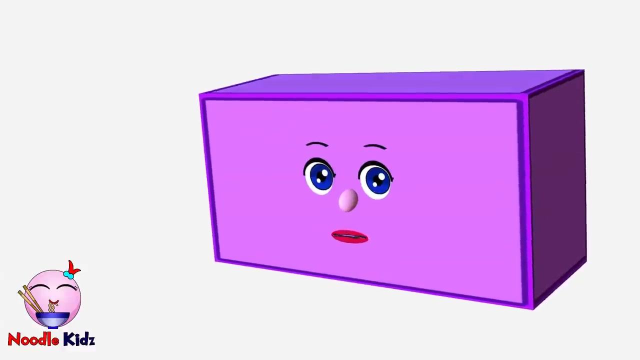 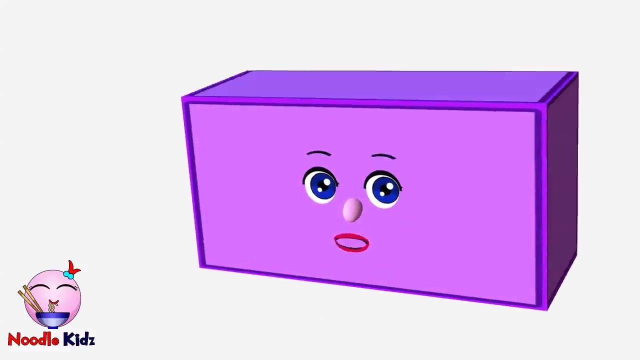 So a cylinder has one curved face, two flat surfaces, zero edges. A cylinder has. A cylinder has one curved face, two flat surfaces, zero edges. And I am a cuboid. I look similar to a cube, but a cube has the same length of edges. I have some different length of edges. 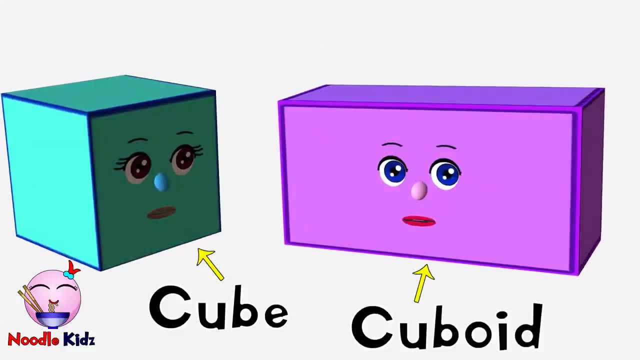 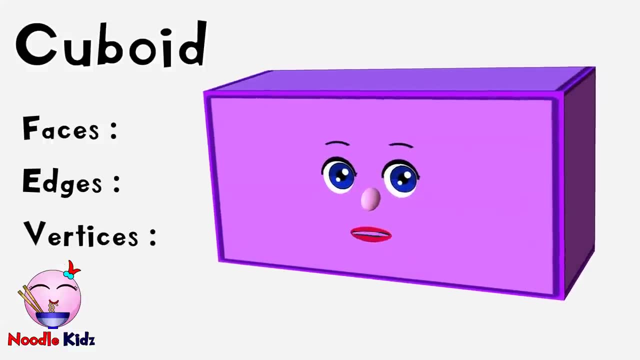 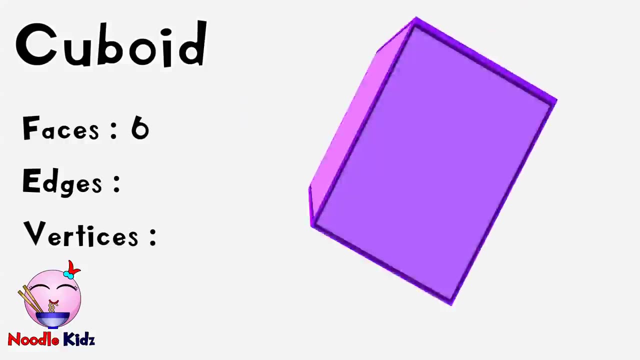 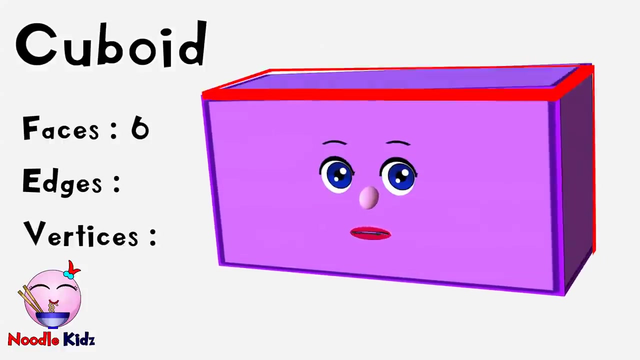 Look at us Cube: Cuboid, Similar but different. right I have one, two, three, four, five, six faces And I have one, two, three, four, five, six, seven, eight, nine, ten. 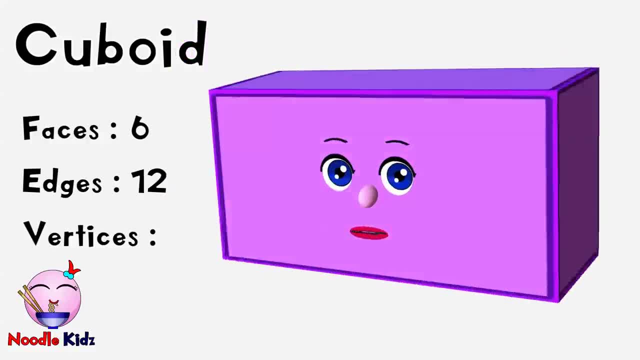 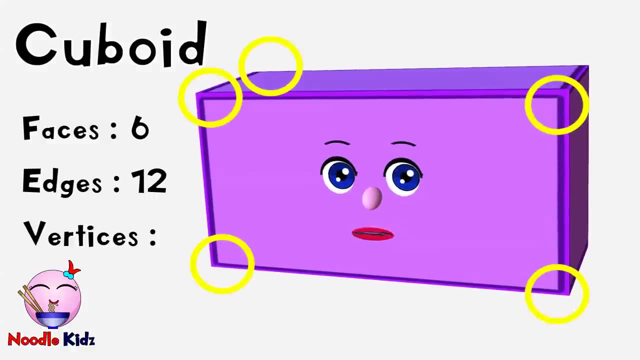 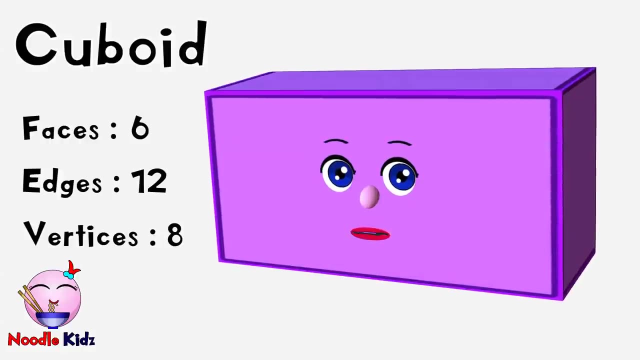 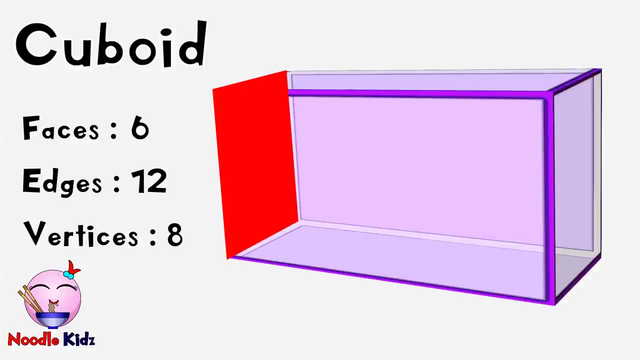 11,, 12 edges. I also have 1,, 2,, 3,, 4,, 5,, 6,, 7,, 8 vertices. So, just like a cube, a cuboid also has 6 faces, 12 edges and 8 vertices. A cuboid has 6 faces, 12 edges. 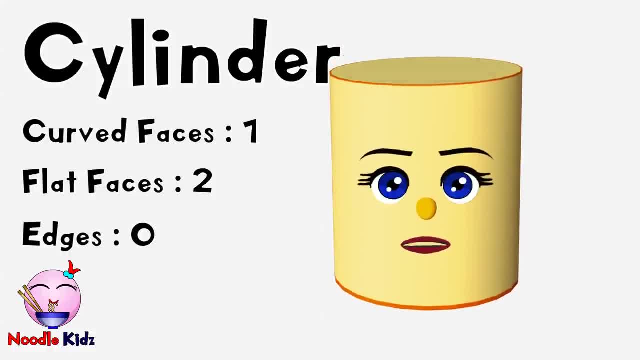 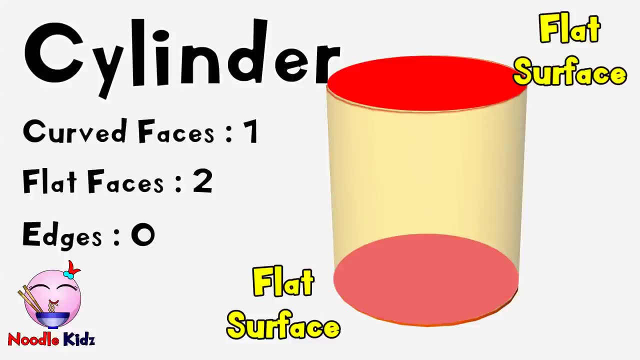 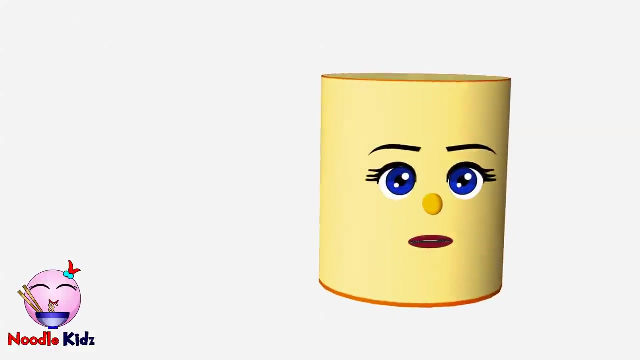 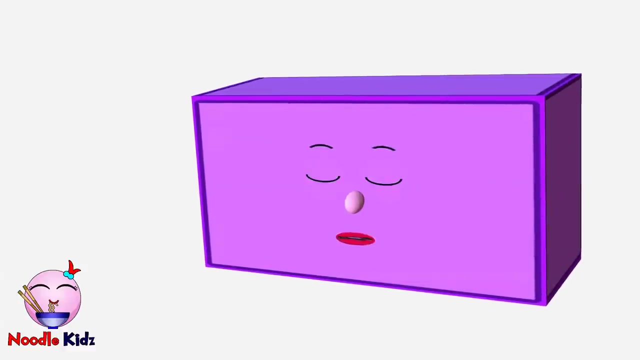 which means I also don't have any vertices. So a cylinder has one curved face, two flat surfaces, zero edges. A cylinder has one curved face, two flat surfaces, zero edges, And I am a cuboid. I look similar to a cube. 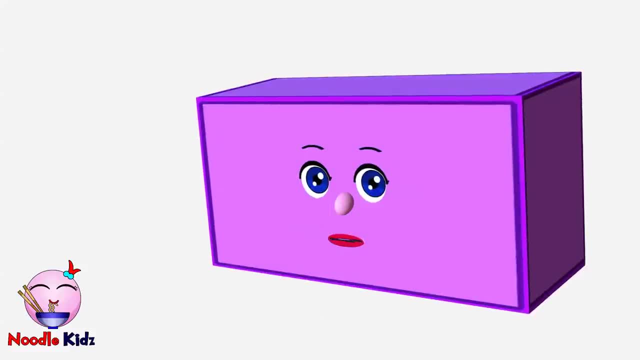 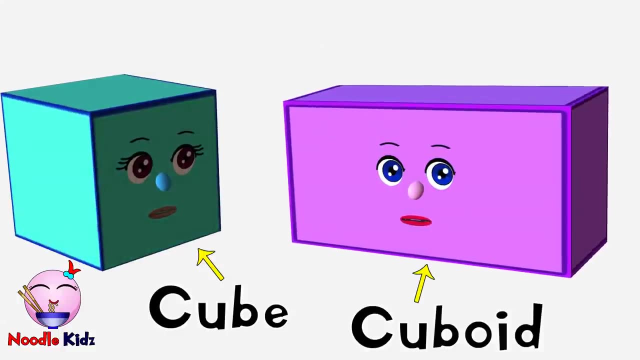 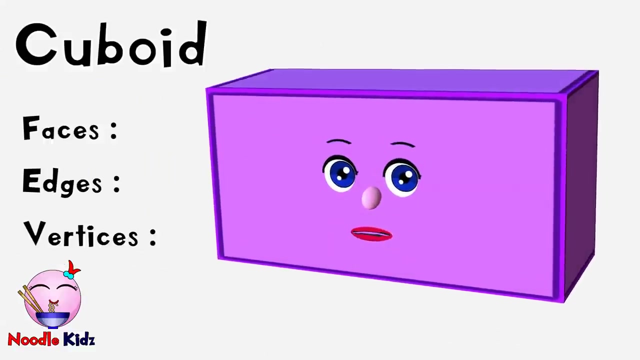 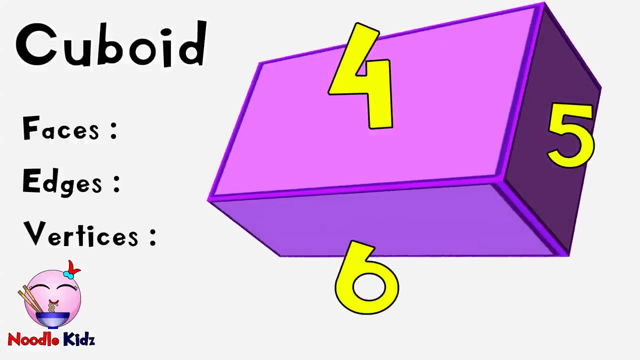 but a cube has the same length of edges. I have some different length of edges. Look at us, Cube, Cuboid. Similar but different. right, I have one, two, three, four, five, six faces and I have one, two, three, four, five. 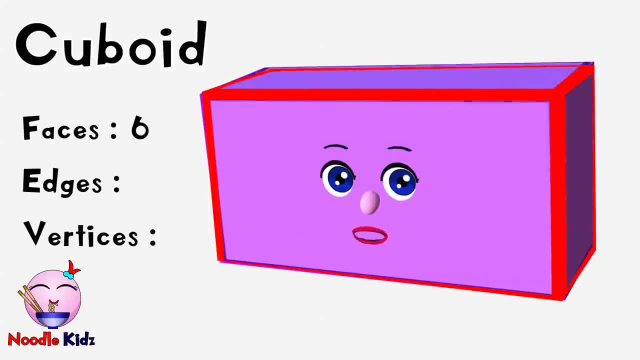 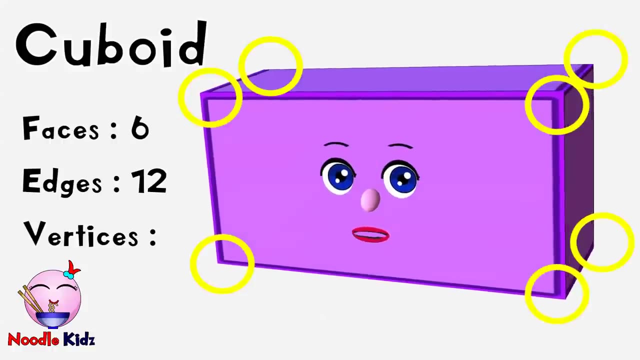 six, seven, eight, nine, 10,, 11,, 12,, 13 faces, 12 edges. I also have 1,, 2,, 3,, 4,, 5,, 6,, 7,, 8 vertices. So just like a cube, a cuboid. 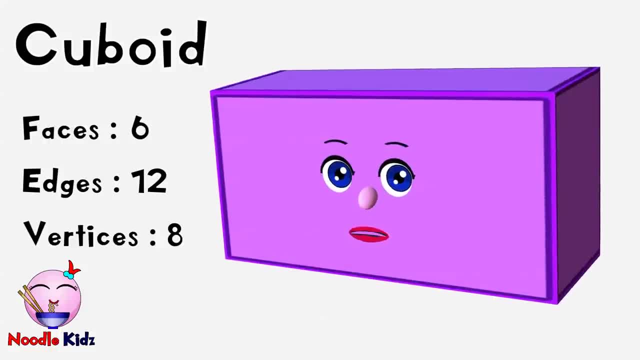 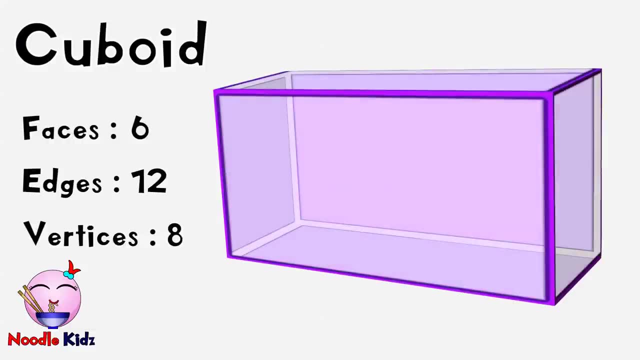 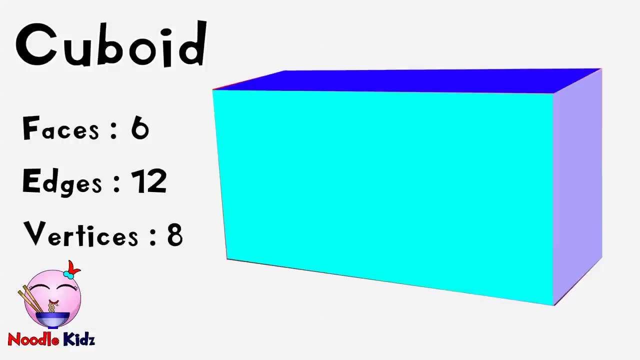 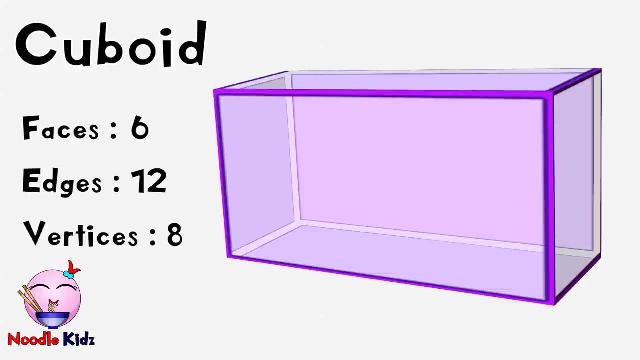 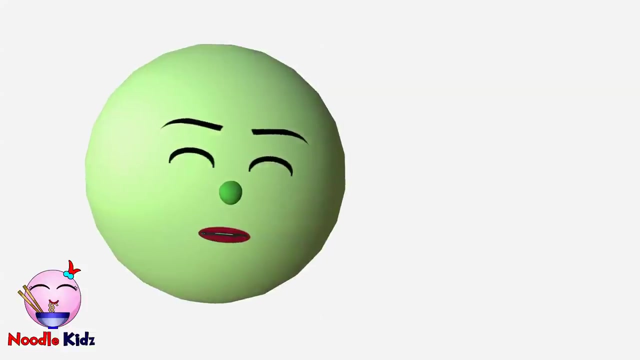 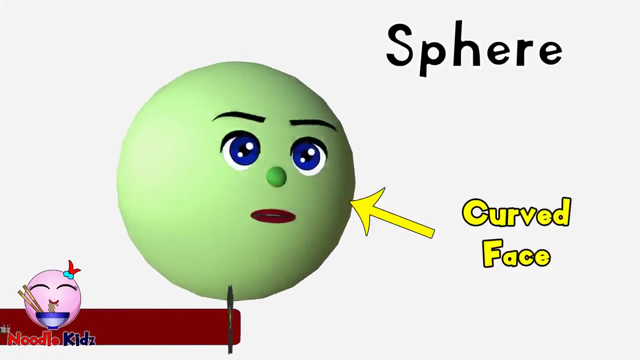 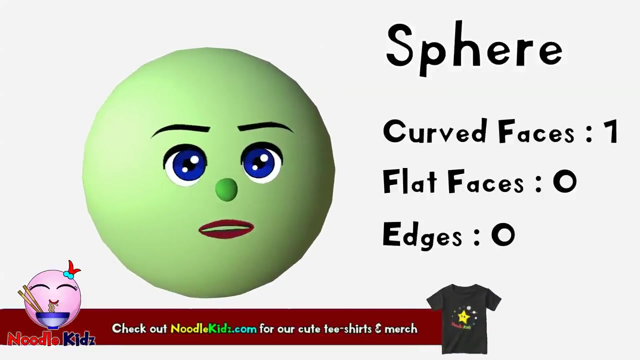 also has 6 faces, 12 edges and 8 vertices. A cuboid has 6 faces, 12 edges and 8 vertices. I'm back. Let's count how many different flat surfaces I have. Yeah, I have 0 flat surfaces, which means I have no edges nor vertices. So a sphere.